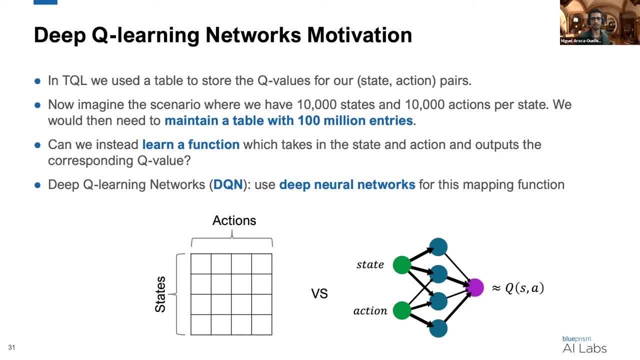 allow us to handle, you know, state and action spaces of a much larger size. And that's exactly the idea behind DQNs, where, for this mapping function, we'll be using a deep neural network. So, as shown in the bottom left, here we have our state, we have our action. it's going to pass. 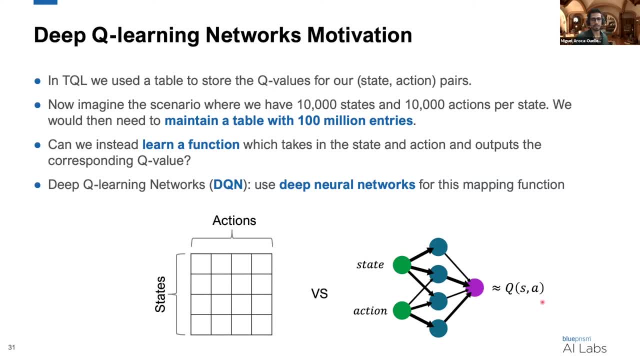 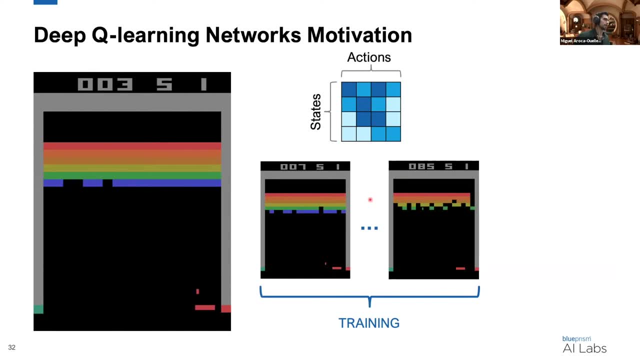 through a network and we're going to get a Q value for that state and action. Another motivation for DQNs is: you kind of be seen in this example here. So on the left here we have this: A, we have an agent who's playing the entire game Breakout And as he's playing he's collecting. 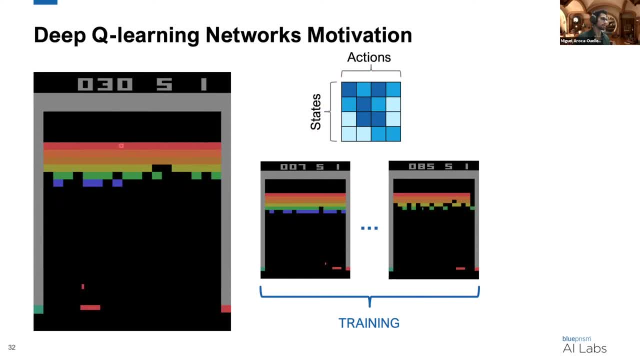 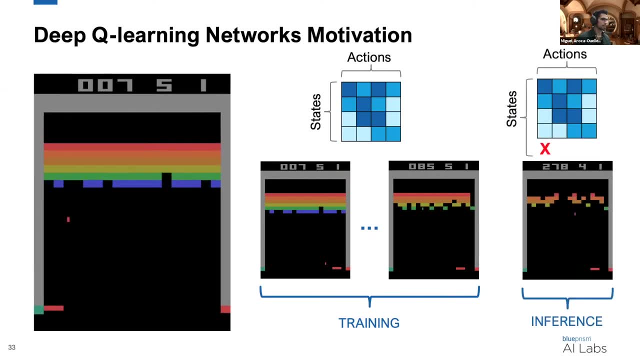 training data and filling in his TQL table. So this is our TQL approach here. However, what happens if, during inference, we all of a sudden see a state that we didn't see during training? So if it's not in our Q table, what do we do? Do we maybe randomly pick an action for that state? 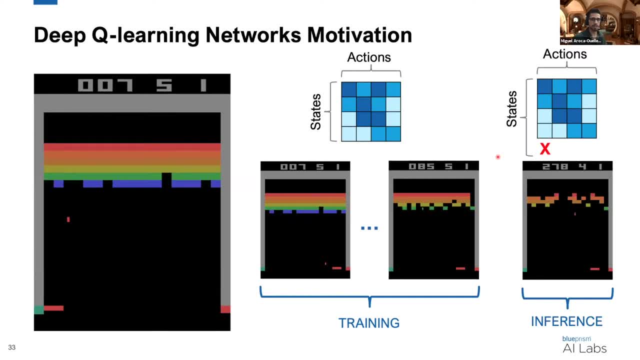 try to find a similar state. Well, this is kind of one of the big downsides of TQL which using DQN can solve. With DQN, we can still apply our QNetwork on these unseen states, as we have on the right here. 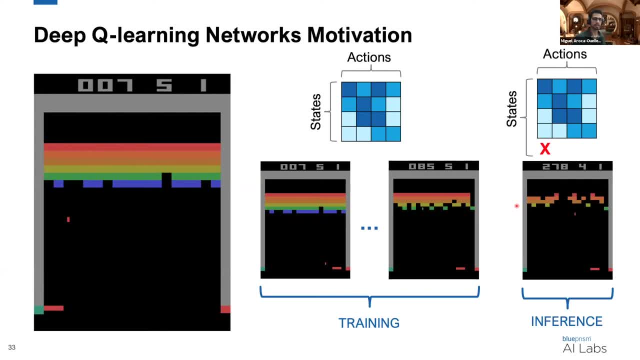 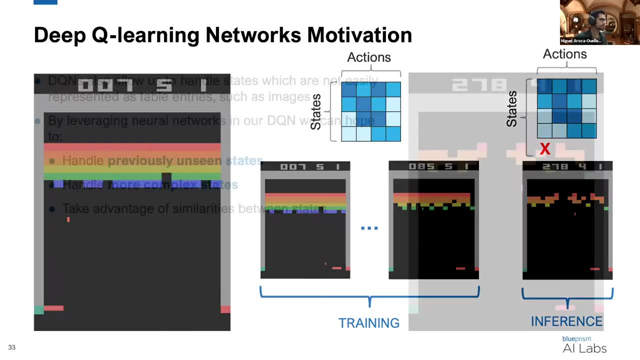 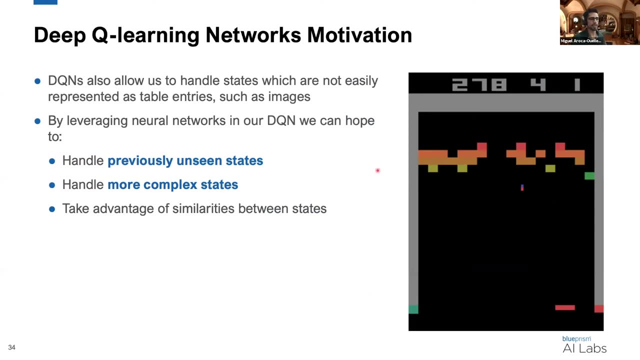 And if our QNetwork is well-trained, it should be able to generalize to these states quite well because of the similarity to maybe previously seen states. Furthermore, DQN allows us to handle states which don't really fit nicely into a table. So in our frozen lake example, we had this grid. 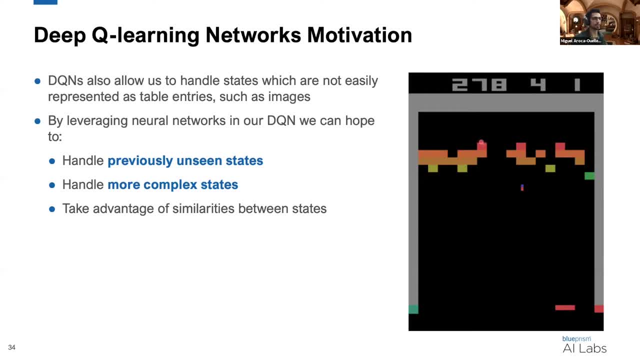 So it was easy to translate this grid into table entries with our actions. But in this breakout game example, it's not necessarily clear how we would actually take this image and put it into a table. Perhaps we could hash it, and there's definitely. 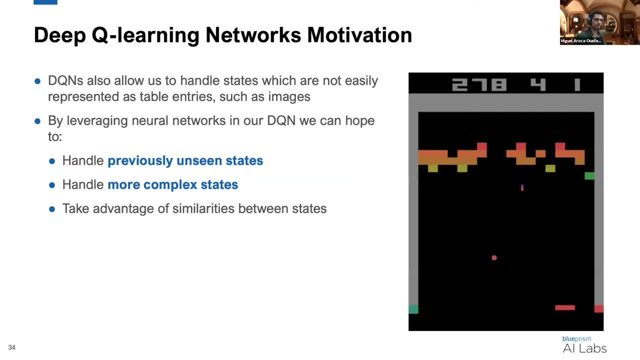 some workarounds, But it doesn't. It's just naturally a map, And even if we did hash it we would be losing some information. Since DQNs use neural network, we can kind of build off all this work on computer vision, which neural networks have. 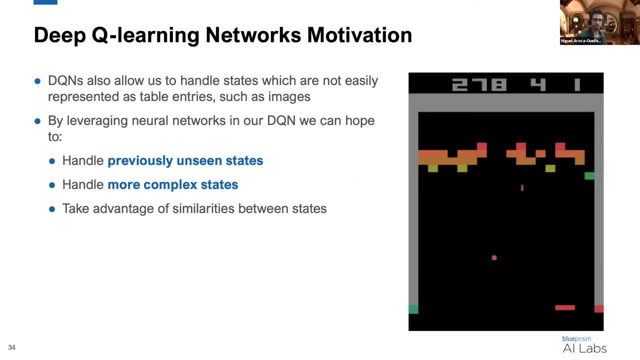 had a lot of success with, And this allows us to handle much more complex states as well as states we haven't seen before, And hopefully, if our network has been well-trained, we can take advantage of these states And we can see the similarities of our states. 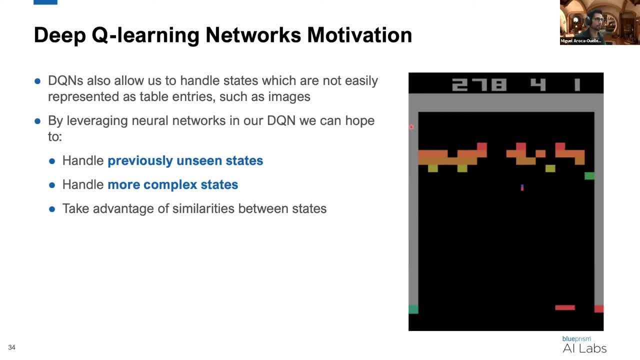 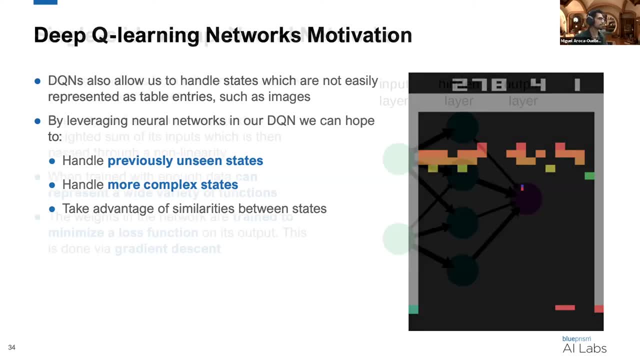 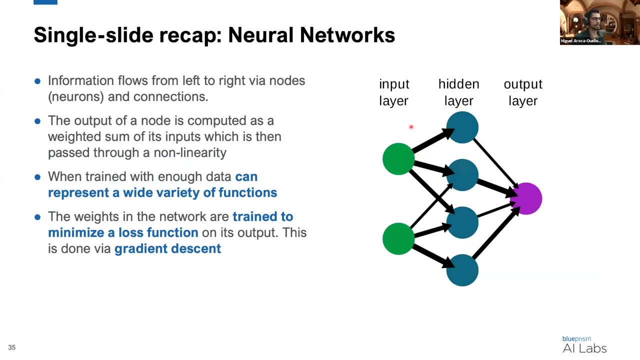 Our network kind of works as a feature extractor And we will potentially perform quite well on states we haven't seen before if they are similar to states we have seen. So unfortunately I don't have time to go into the details of neural networks in this tutorial. 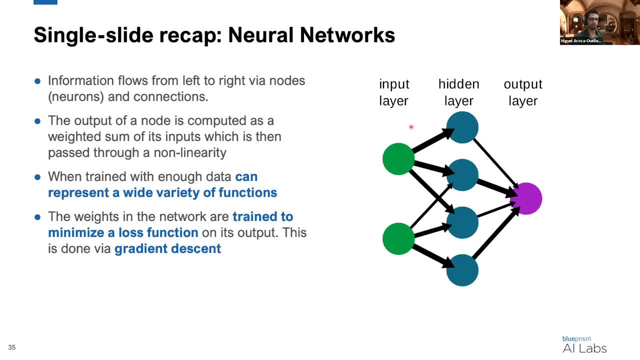 And I'm sure many of you are familiar with them already, So I'll give a very quick one slide recap for those who aren't familiar. As the name might suggest, they're motivated by the idea of neurons in biology, And what we have is we have these different nodes. 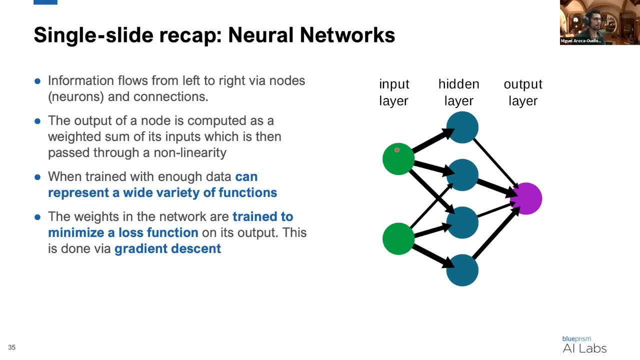 as we see in this diagram here, And these nodes compose different layers which take in information from the previous layer through these arrows. sum them up, sum up their inputs and pass them through a non-linearity to the following layer, And the way that we train them is. 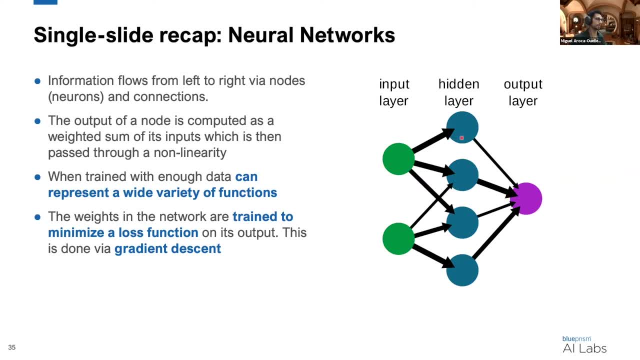 simply by doing this, By training these weights connecting these different nodes, And we train them by minimizing a loss function on the output, And this is done via gradient descent. It's been shown that neural networks can approximate a wide variety of functions, which 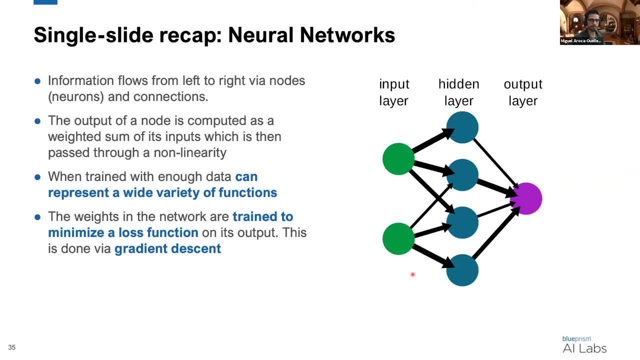 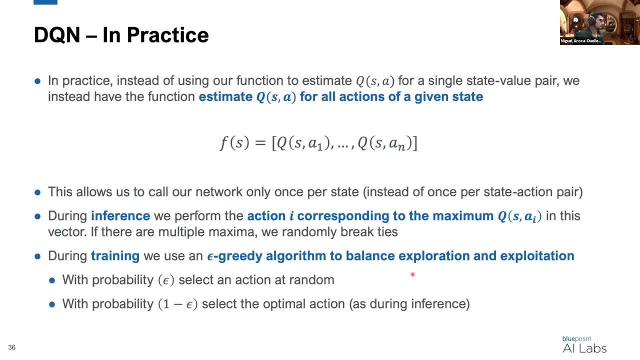 allows us to do quite well in a lot of settings. So one quick twist to what I said previously: In practice we actually don't take in the state and the action as inputs. What we do is we actually simply take in the state and then output a vector of Q values for all actions. 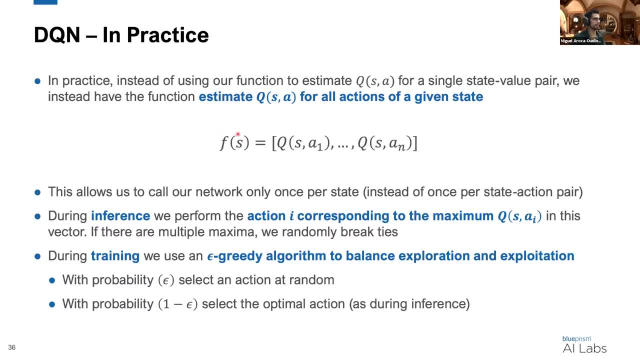 And this is represented in this equation here. So we take in the state in our network and we output one Q value for each action. And the reason we do this is that it allows us to call our network only once per state instead of once for every state action pair. 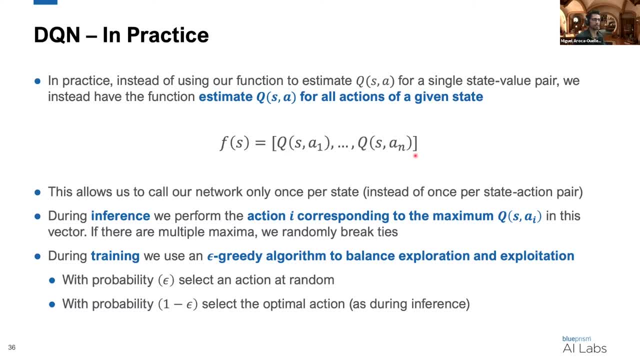 And that's why we do this. It lets us take advantage of the potential parallelism During inference, when the agent is actually being evaluated. it selects the action which has the highest Q value from this vector And, if there's multiple maxima, you. 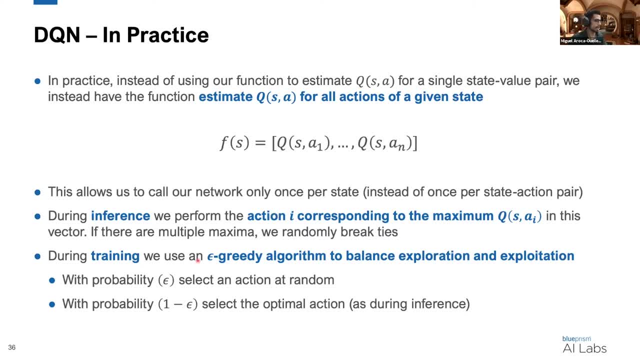 can simply randomly break ties. And then during training we encounter this issue again that John presented previously, this idea of balancing exploration and exploitation, And here what we do is we use an epsilon greedy algorithm to balance it. So during training, with some small probability, epsilon 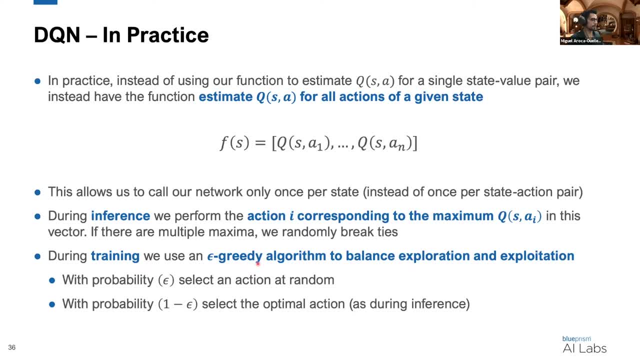 we'll select an action at random And then, with probably 1 minus epsilon, we select the optimal action, as we are doing during inference, And this allows us to exploit actions we know do well during training, so, for example, not falling into an icy hole while still allow. 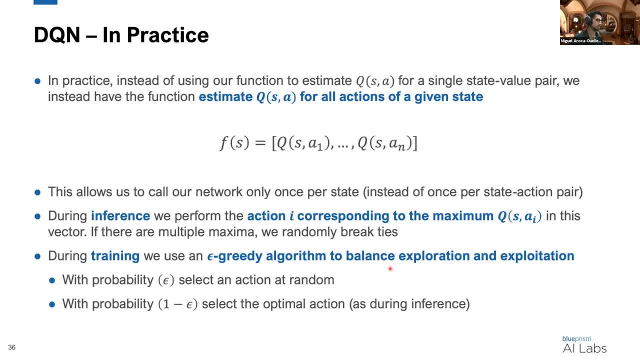 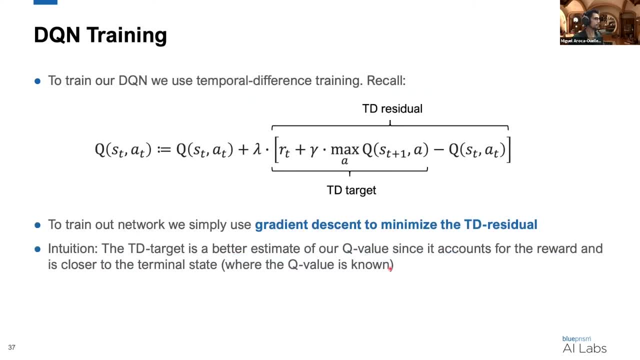 us to explore new actions which might lead to better rewards in the future, so traveling around our lake, for example, to try to get to the goal. So once again, we have our Q learning equation here, where we have our new Q values, which are updated. 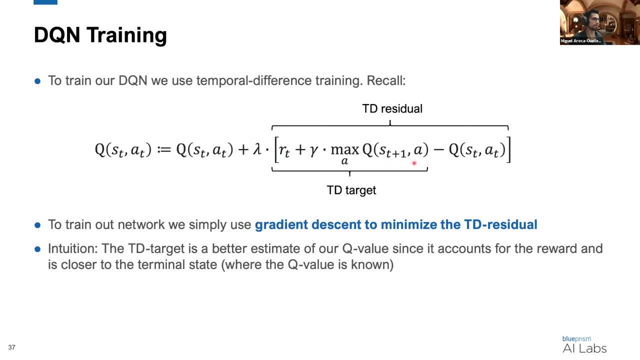 based on a learner rate, our TD target, which is composed of our reward Plus our discounted future Q value here, as well as our Q value for the current state in action. And our goal here is we want to train our Q network to optimize, to minimize this TD residual. 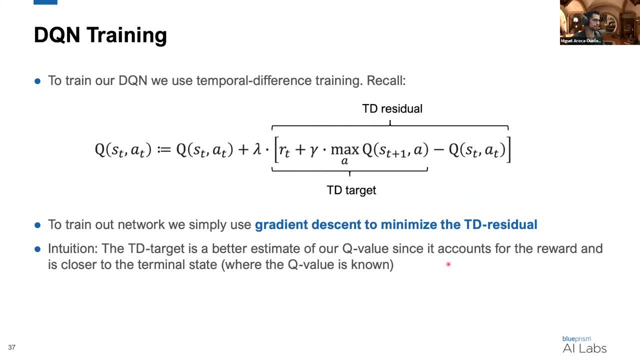 So we're going to use gradient descent to minimize this TD residual And, as John mentioned previously, the intuition here is that our TD target this term, with the reward and the maximum action, is a better estimate of a Q value because A of course it already accounts for the reward. 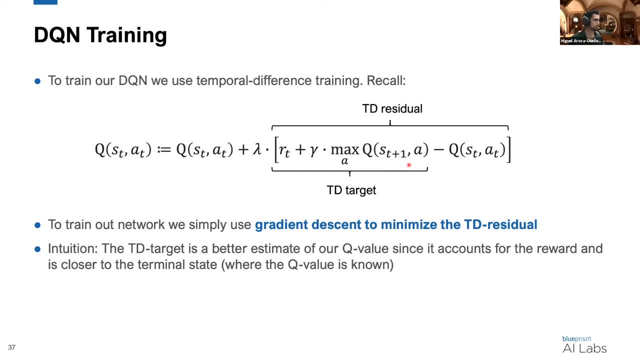 that we are getting by selecting this action, But also it's also closer to the terminal state, where we do in fact know the Q value, since that's where we'll be receiving our reward. So we're trying to move our current estimate. 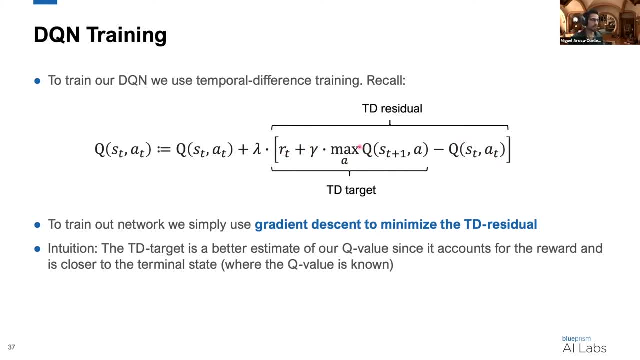 towards this future more accurate estimate In the simplest setup we can do this. We can do this Q-learning update at every time step, But we could also potentially batch the updates, which might help with the stability And if you are familiar with neural networks. 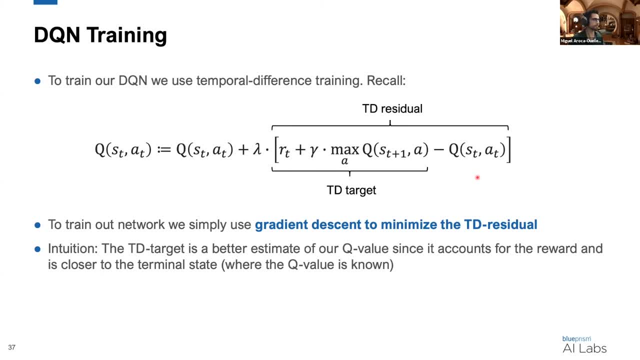 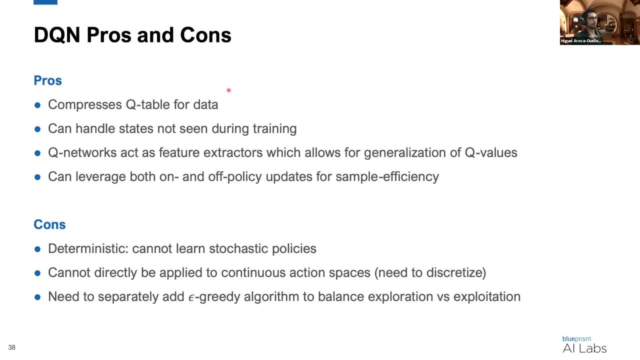 you will be familiar with the concept of batch updates. So, to summarize a couple of the pros and cons of DQN- And this will kind of motivate as well some of the other approaches in reinforcement learning that we will be talking about later- 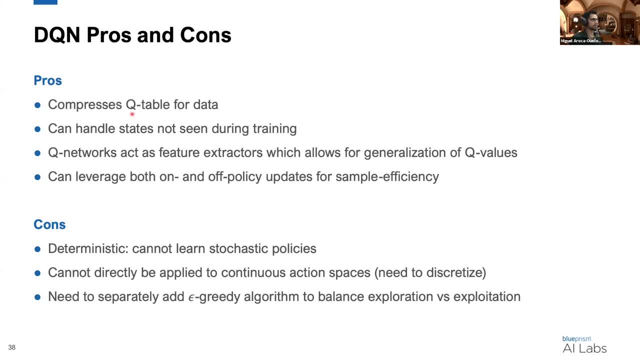 The DQN approach. It can be kind of seen as compressing the Q table down. Instead of having to maintain this large, potentially very large Q table, we can use a network to get our Q values, which allows us to represent a much larger state action space. 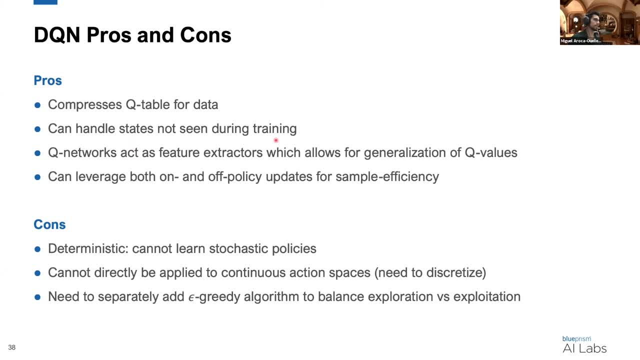 It allows us to handle states not seen during training, as we saw with the breakout example, And the Q network can also be seen as a feature extractor which allows us to generalize to these Q values we haven't seen before And actually do quite well. 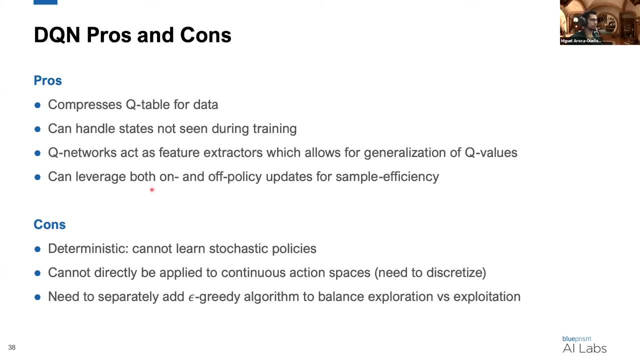 And one more thing to note is that it can leverage. we can learn both on and off policy. So we'll see this in a couple of slides, But we can revisit some of the transitions we saw previously and use those to learn on, So we can train on these off policy examples. 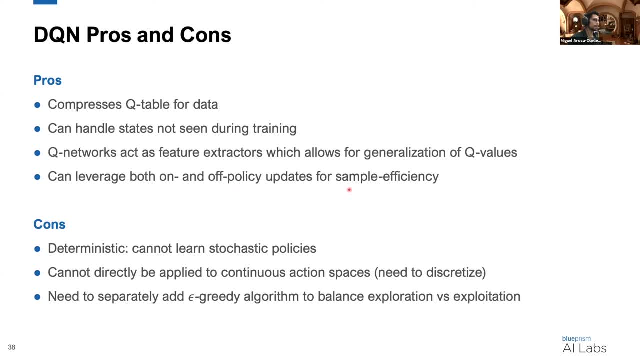 And that allows it to be a lot more sample efficient. And this is a big advantage compared to policy gradient, which we'll be discussing later, Because in policy gradient you can only learn on policy. So by allowing us to learn both an on and off policy- 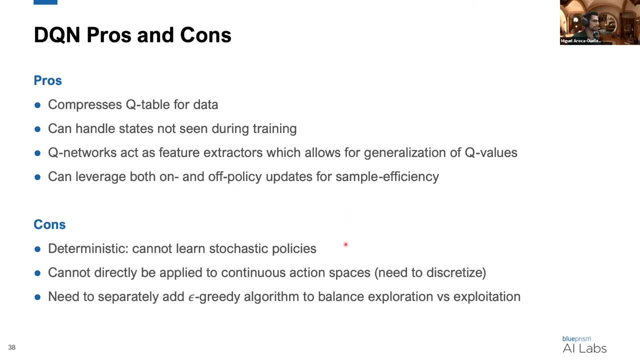 we can kind of take advantage of all these transitions that we've seen. One of the some of the downsides of DQN is that, just like TQL, it still can't deal with stochastic policies. Everything's deterministic. We're taking the maximum action when 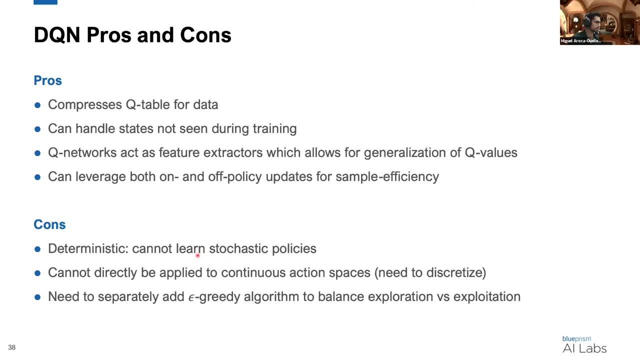 our agent is interacting with the environment and being evaluated. It also can't be directly applied to continuous action spaces. We could kind of get around this by discretizing the continuous action spaces, But in certain instances that may not be what you want to do. 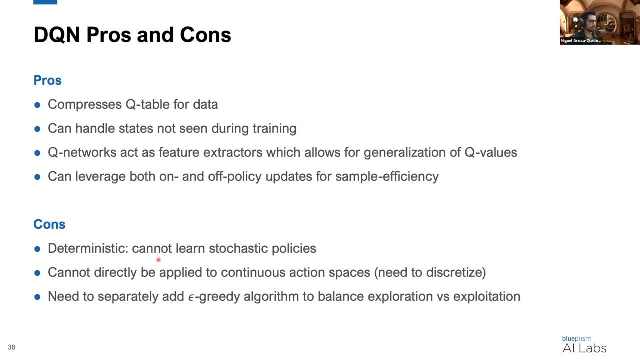 And you'd want to deal with a continuous action space directly, And DQN simply can't do that. And then, finally, as I mentioned, we need to separately have this epsilon greedy algorithm to balance exploration versus exploitation, And it would be nice if we could have 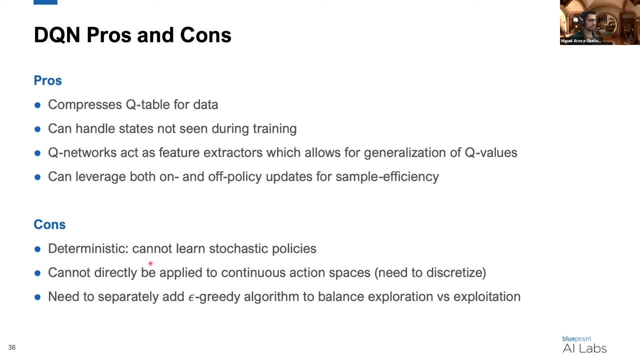 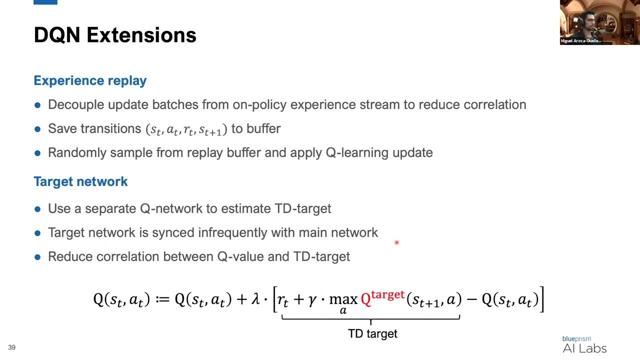 our wish list for our ideal model, if this exploration exploitation balance was actually implicit in the model and we could take advantage of this concept of action uncertainty, as we are learning and interacting with the environment. So that's the basic DQN setup. There is a couple extensions that I'll briefly discuss here. 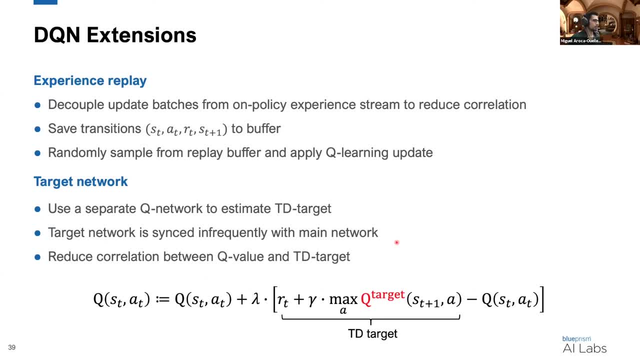 because they do come up in the exercise. So one of the extensions is called experience replay And the idea here, The idea here is you decouple your batch updates of your model from your experience stream. So how that works is that as you interact with the environment, 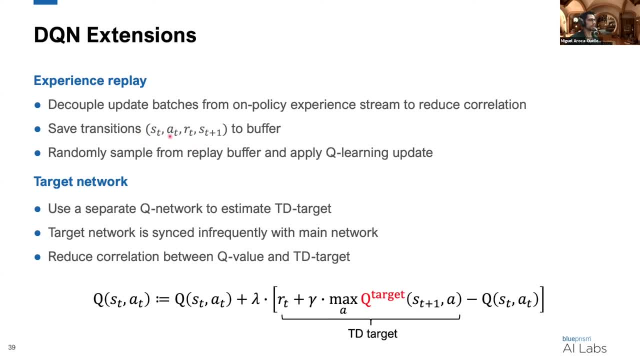 you save your transitions, So a tuple of state, action, reward and next state, And you take that tuple and you store it into a memory buffer And then, when you want to update your model, you'll simply randomly sample from that replay buffer. 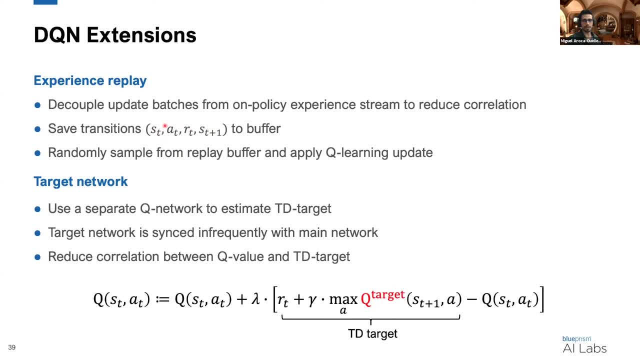 and apply your Q-learning update And this can help a lot with this. So this is a really useful tool to use for understanding the stability of the training, because you're reducing the correlation between all the items in your batch because they're sampled from the memory. 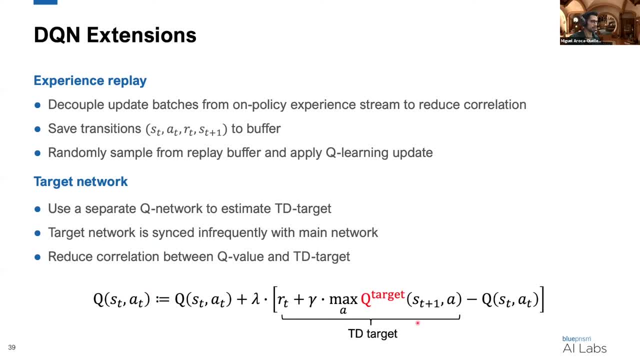 Another improvement is target networks. So the idea with a target network, if we look at this equation on the bottom here, is that in your TD target, instead of using your Q-network, your normal Q-network, which we'll call the online network, you're 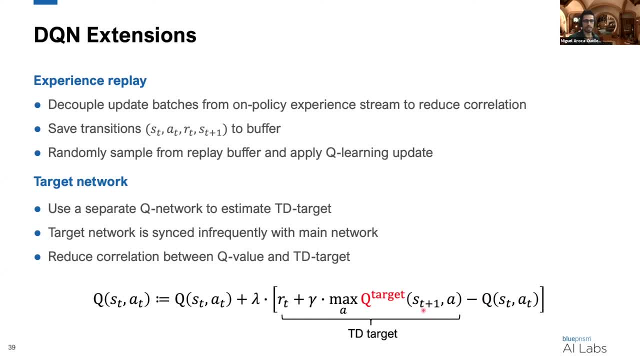 going to use an additional Q-network called the target network And you'd like to do that. is that in the standard approach, this target, because it also is dependent on this Q-network, it's kind of a moving target. You're updating your Q-network and that. 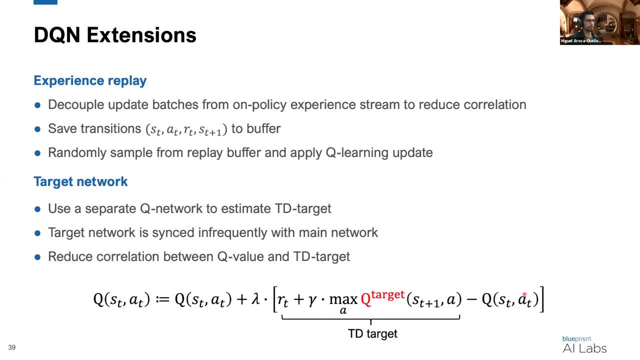 changes both your value- this right value in the residual- but it also changes your target. So you're chasing this moving target, which can make it difficult to learn and quite unstable. So the idea here is you, You actually create a second Q-network here. 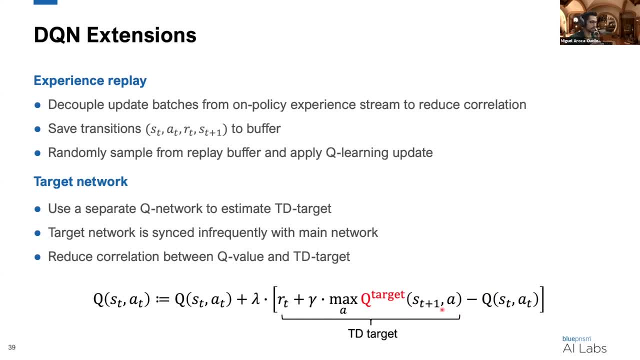 this target network and that kind of stabilizes your goal and really kind of stabilizes the training. So you have two networks. You have the target network, the online network. The online network you update as usual, as we saw before. 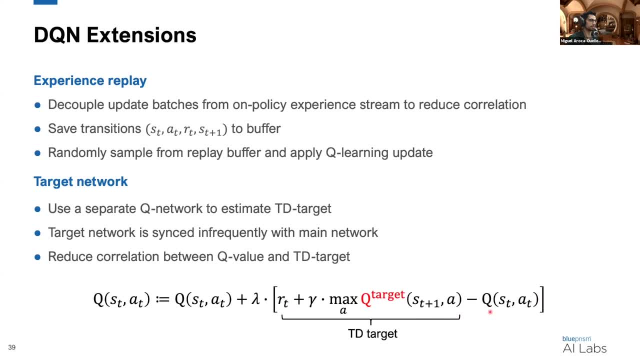 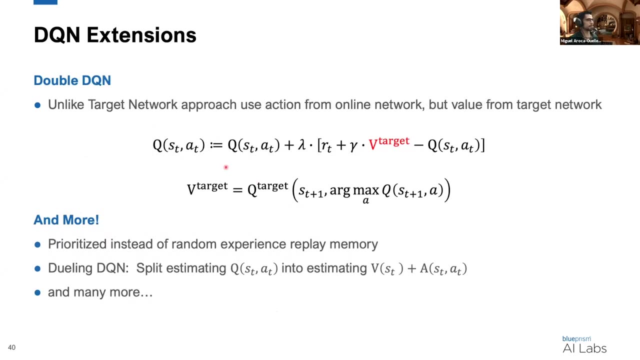 And then this target network. you infrequently update it. based on this online network, You're going to kind of copy over all the weight values every once in a while to update it. So, in that same vein, and there's this idea of double DQN- 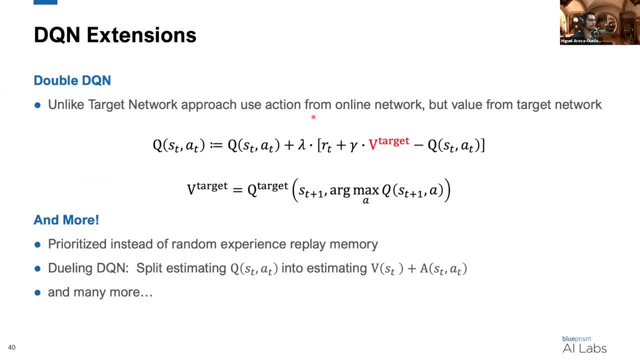 So double DQN builds off this idea of a target network, except that instead of using the target network to select the value- sorry, to select the action- you'll be using your online network to select the action. So you select the action with the online network. 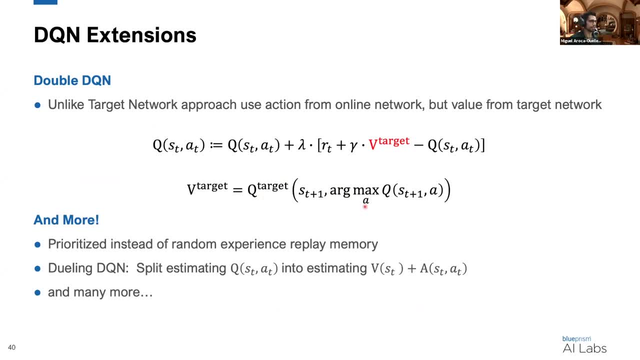 You pass it through the target network to get your target Q-network And then in turn, the action routes will not manera that, but you- classic resonance decreasing of the action- encont Hasta the visual of the target network and the operating agreement. So the action process begins with the Q value. 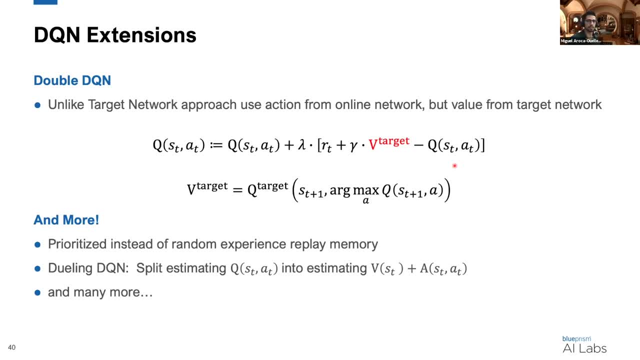 and then you update as normal. So this decoupling of the at this full decoupling of the action selection and the evaluation helps kind of reduce these estimation issues with the Q values and once again kind of leads to more stable learning. 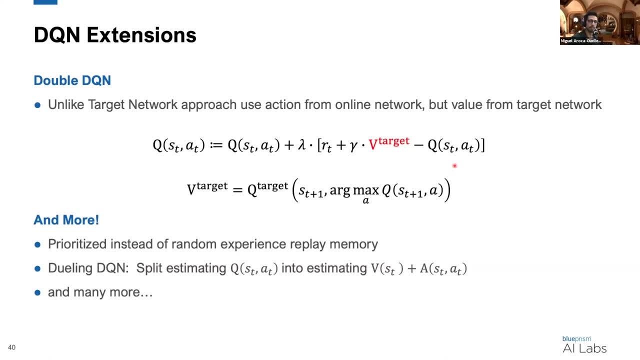 so kind of. all these extensions are really focused on improving the stability of the DQN approach, And then, of course, there's a bunch more work that's been done in this to improve on this, this amount of randomness and performance approach. on these basic dequeuing approaches, We can use prioritized replay, So instead of randomly. 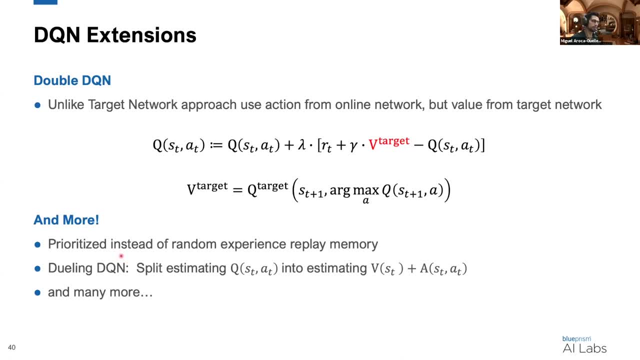 sampling from our replay memory. we can prioritize certain memories. So, for example, if some of the transitions that we saw have a very high TD residual, we could say that those transitions are potentially more useful to learn from than those where we're doing a very good job of. 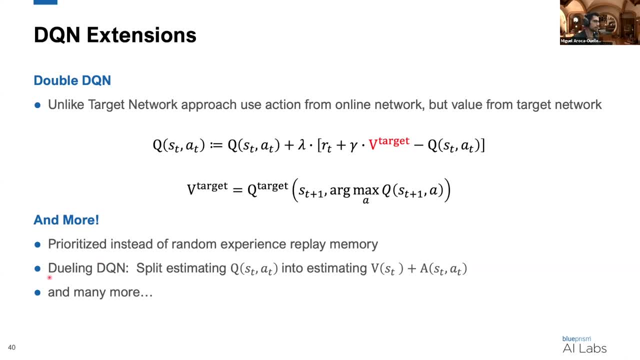 estimating dequeue values. already. There's also another extension similar to double dequeuen, where it's called dueling dequeuen, And there's a little bit sometimes of confusion in the literature here because they both get abbreviated to DDQN. But the idea here is you split your. 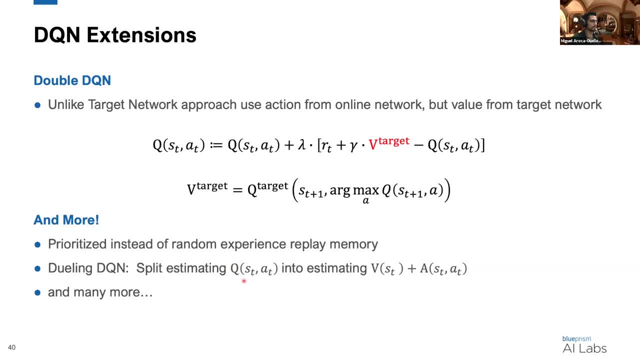 estimate of the dequeue value into two parts. Instead of estimating just the dequeue value, you estimate the value of the state As well as the advantage of taking an action given that state, And this will actually come up again in the discussion on actor critics, where you have this idea of a state baseline. 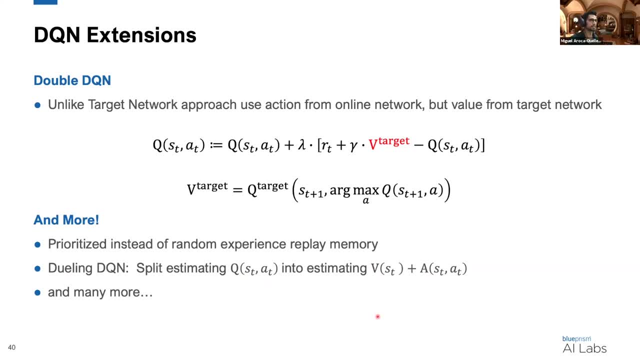 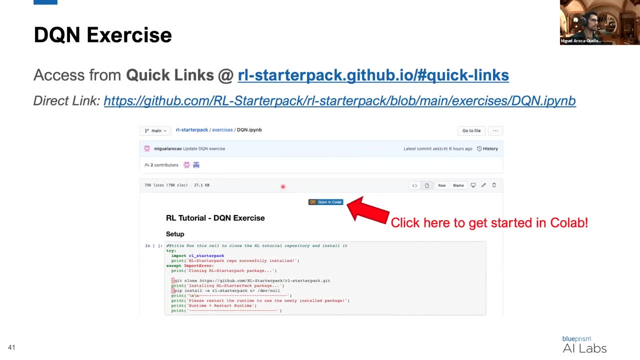 And this helps with the variance of your updates. Okay, so that leads us to the next exercise, So you can follow the quick links on the screen. I'll put the link in the chat box. Okay, so that leads us to the next exercise, So you can follow the quick links on the screen. 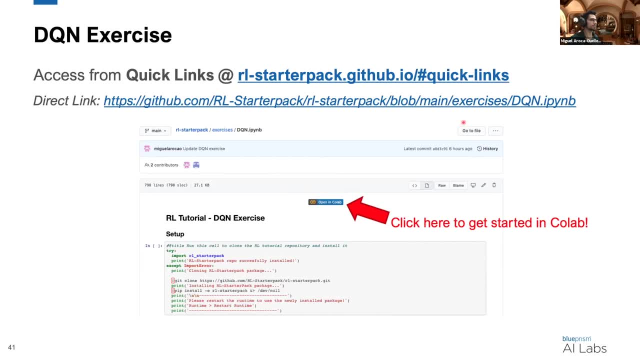 Okay, so that leads us to the next exercise. So you can follow the quick links on the screen. Okay, so that leads us to the next exercise. So you can follow the quick links on the screen On the website here, or use this direct link which we will post in the chat And similarly. 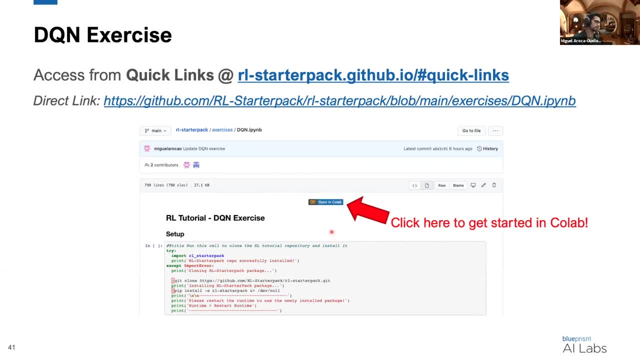 once again, just make sure you open it in COLAB and the setup should be similar to the TQL. There's both the basic dequeuing implementation as well as the experience. replay is also in there, as well as the target network. And, once again, feel free to ask questions in the chat or to 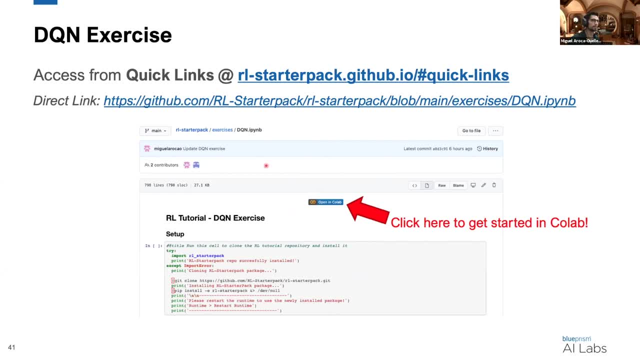 unmute yourself and ask questions, And I think that's enough time. we'll be setting up breakout rooms as well. Thank you. 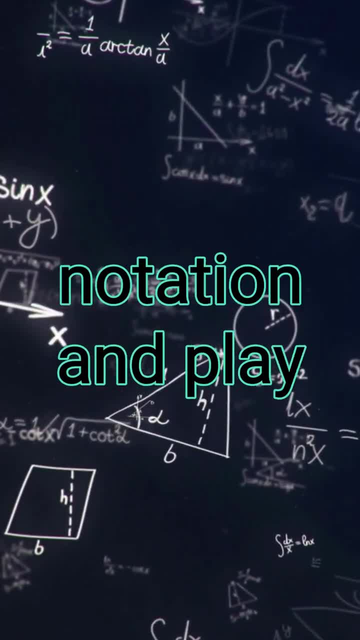 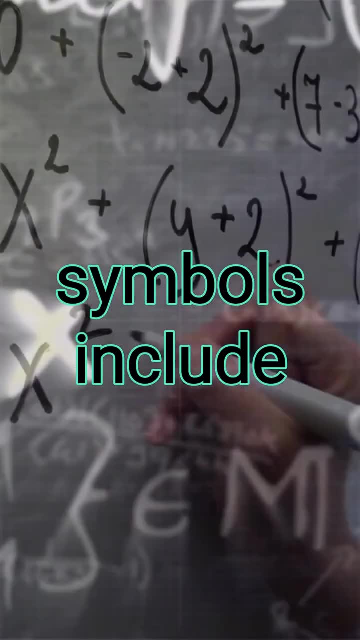 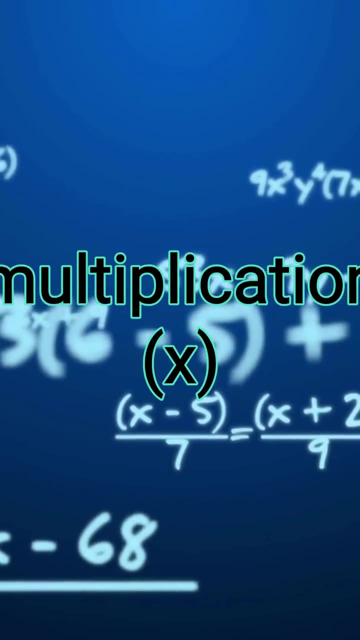 Math symbols are the building blocks of mathematical notation and play a crucial role in conveying mathematical ideas and concepts. Some of the most commonly used math symbols include plus and minus signs, which are used for addition and subtraction operations. Multiplication symbol X, which represents the product of two or more numbers. 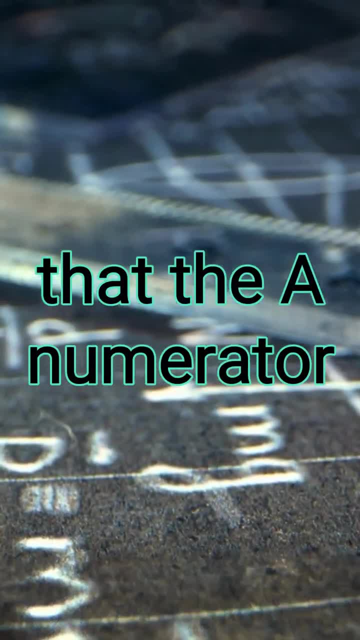 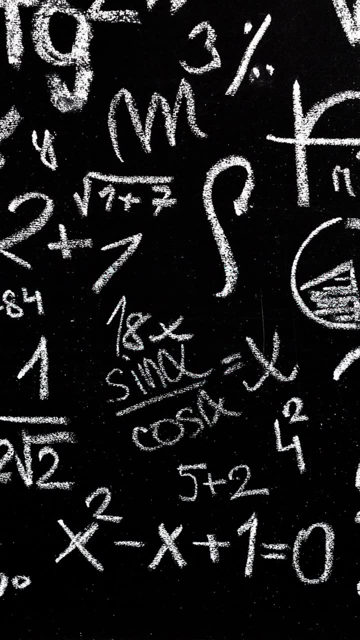 Division symbol. forward slash which indicates that the numerator is being divided by the denominator Equal, equal, sign. sign which is used to indicate that two expressions are equal in value, Greater than greater than sign and less than less than sign. symbols which are used to: